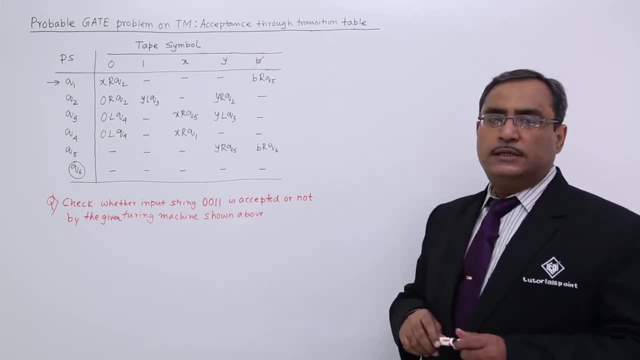 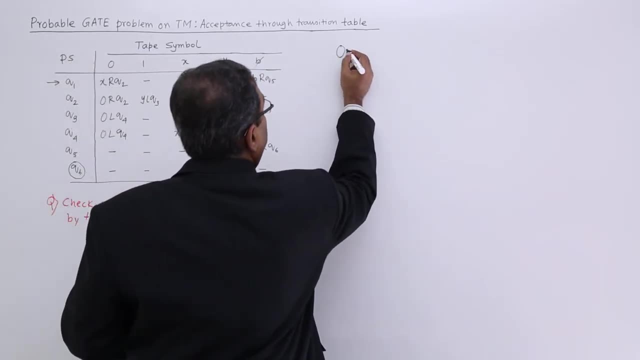 I shall write this instantaneous descriptions in three different notations. You also see that one. Now we are going for the 0, 0, 1, 1.. So 0, 0, 1, 1 is my input string. So I am with the initial state q1.. So that is the transition. 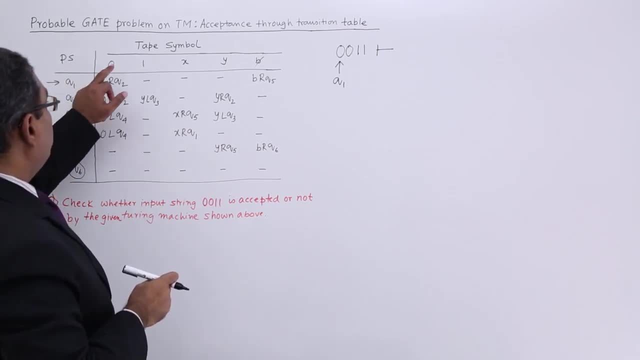 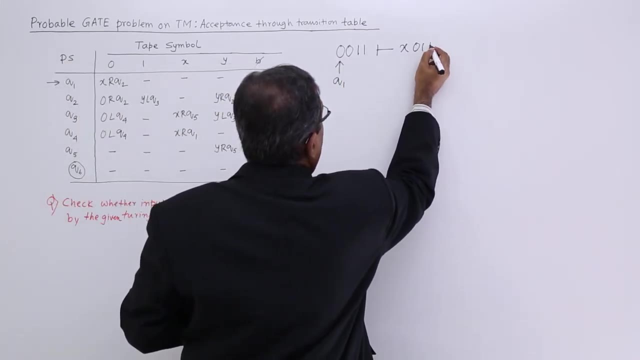 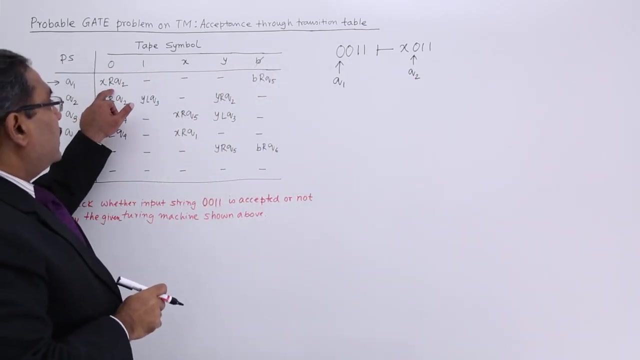 I am going to do Now q1, 0.. q1, 0 is xrq2.. xrq2 means 0 will be replaced by x. I shall move to the right hand side and next it will be q2.. So q1, 0 means xrq2.. So 0 will be. 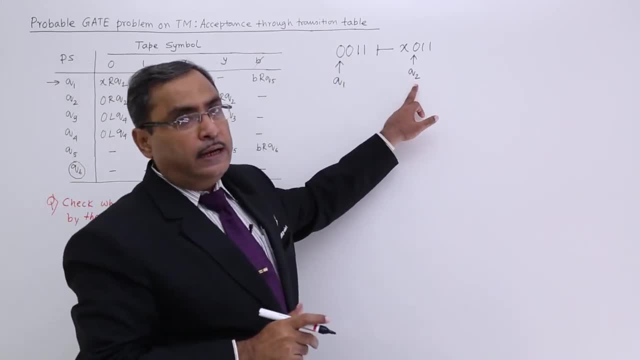 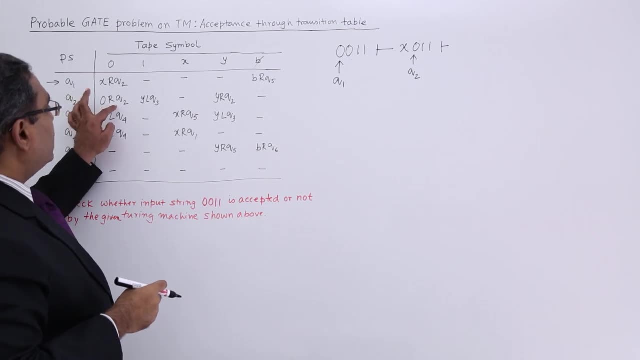 replaced by x, I shall move towards the right hand side. then I will be at the state q2.. Now what about the next? That is q2, 0. So q2, 0.. 0rq2.. q2, 0 is 0rq2.. So 0 will be. 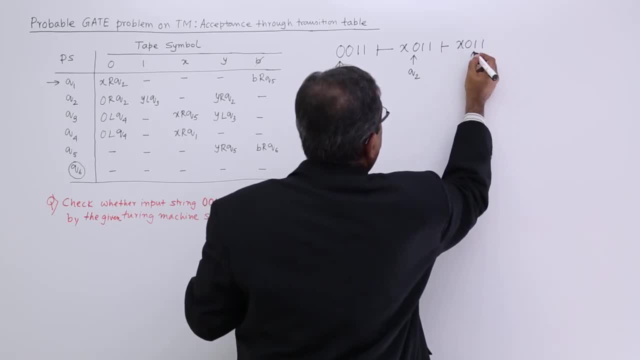 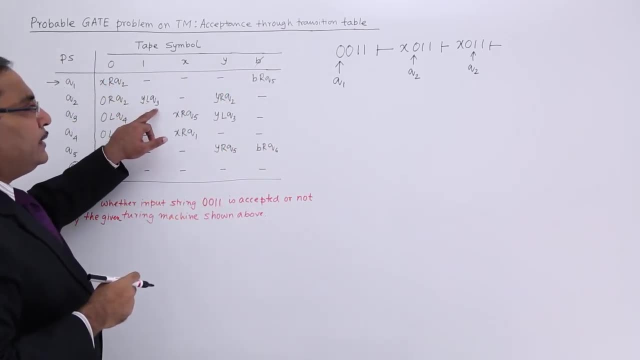 written as 0.. I shall move towards the right hand side. I shall remain with the state q2.. Now q2, 1.. q2, 1.. ylq3.. ylq3.. So x0 will be there. 1 will be replaced by y, 1 will. 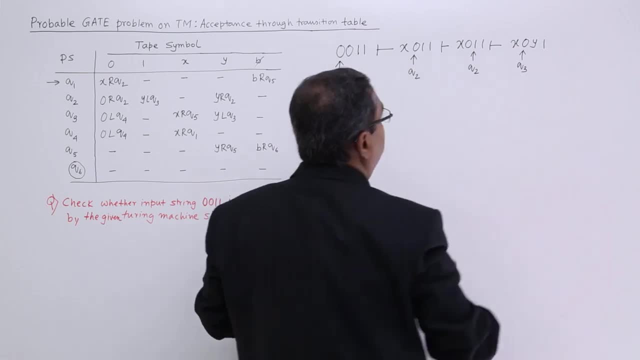 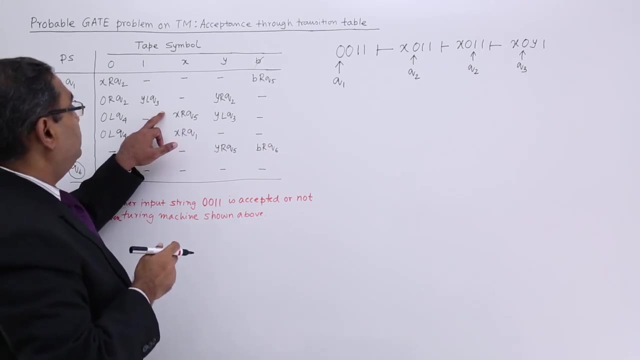 be there. I shall move towards the left and I shall be at the state q3.. So q2, 1 means ylq3.. I have done the same. Now, next one, That is my q3, 0.. Now, next, I shall search. 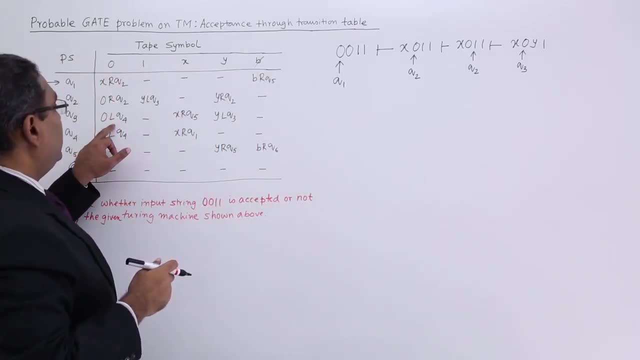 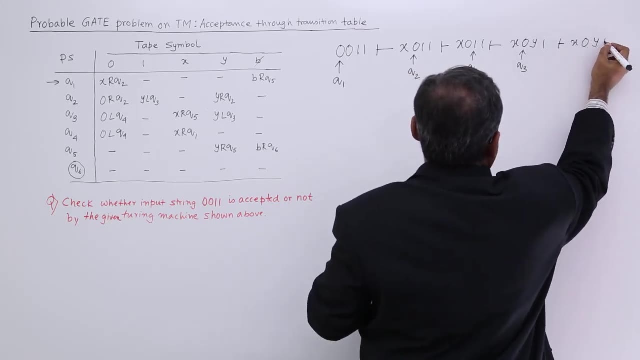 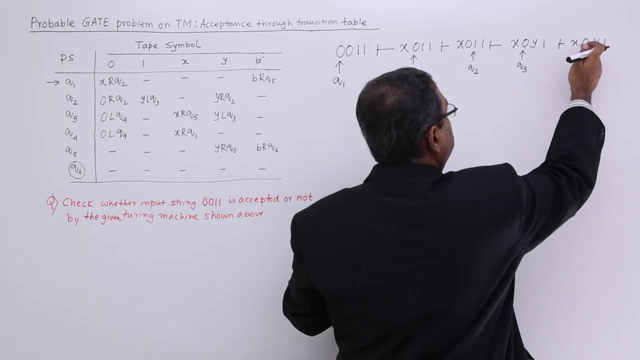 for q3, 0. So q3, 0.. 0lq4.. So now x will be replaced by x will be there. So q3, 0- lq4. So 0 will be written by 0.. I shall move to the left hand side. left left symbol. 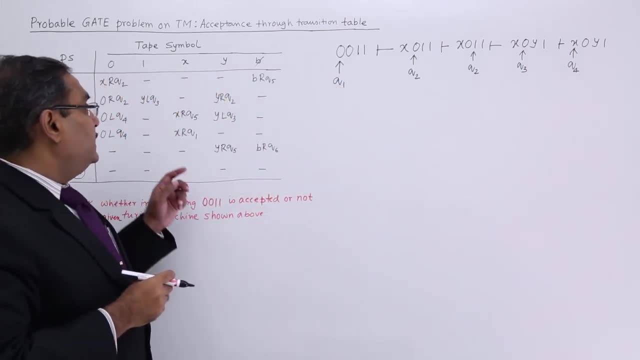 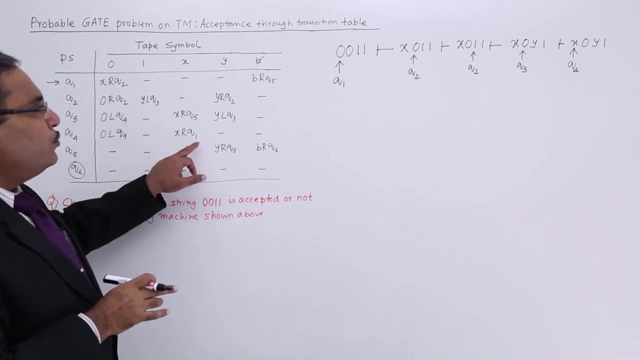 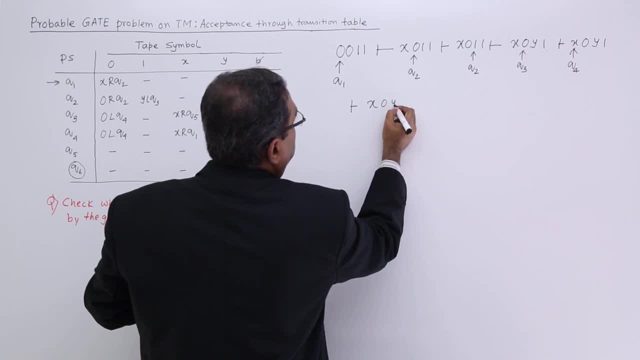 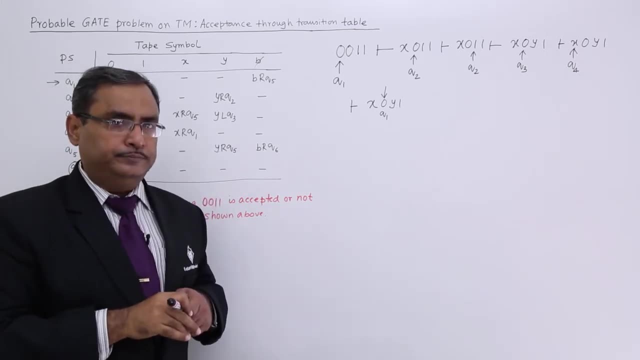 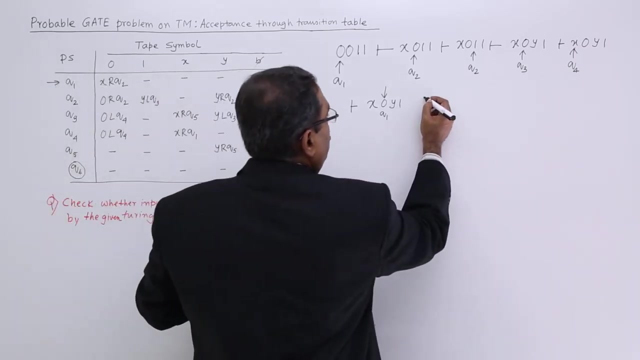 X R Q 1.. So X Q 1 and right hand side. So that is another notation. I am writing Now Q 1: 0.. So Q 1: 0, X R Q 2.. So X R Q 2, 0 will be replaced by X. I shall move towards. 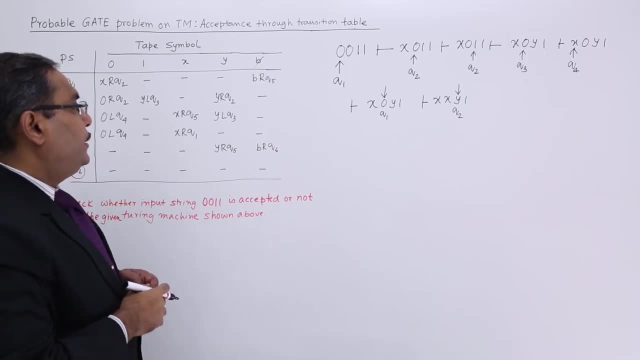 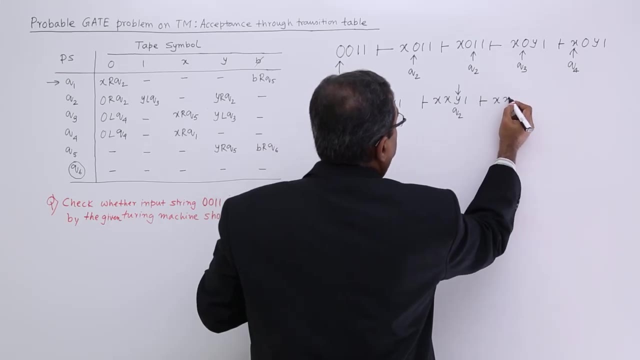 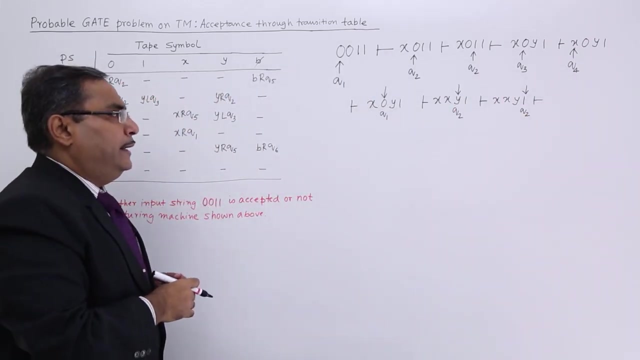 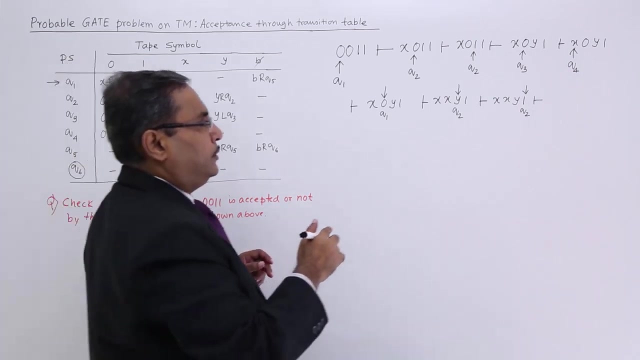 the right, and next it will be Q 2.. Q 2, Y, Q 2, Y, Y, R, Q 2.. So Y will be written as Y R, Q 2.. R means it will move towards the right. Next, that is my Q 2: 1, Q 2 1, Y L, Q 3. So. 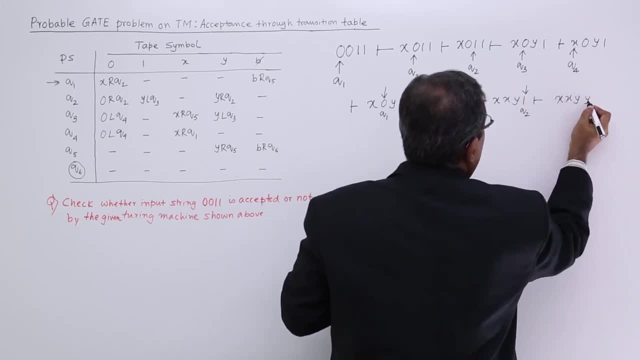 Y L Q 3.. So I shall go for Y. This one will be replaced by Y. So Y L Q 3.. So Y L Q 3.. So I shall go for Y. This one will be replaced by Y. 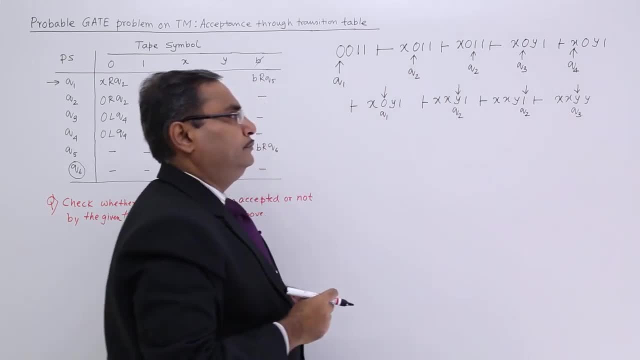 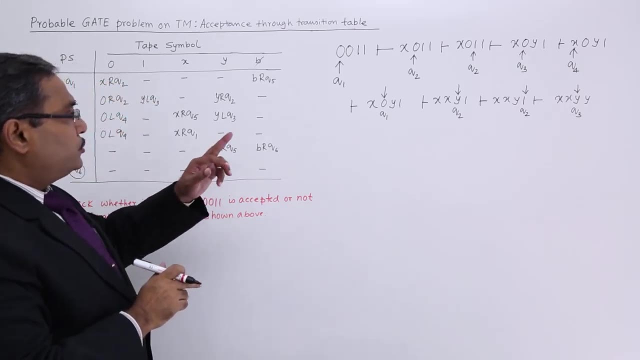 L, and that will be my Q 3.. Next line I shall write in another notation, See Y L, Q 3.. So I have written this one: Q 2 1, Y L, Q 3.. I have written that one. Now next one. Next. 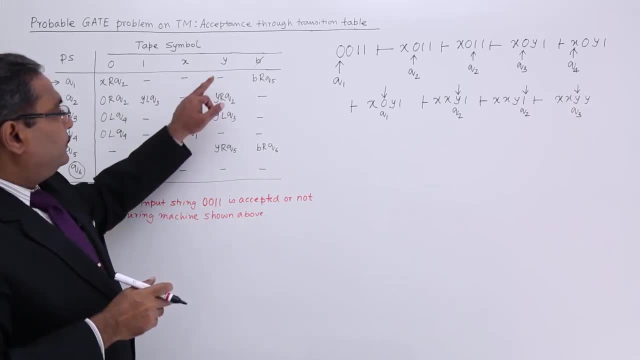 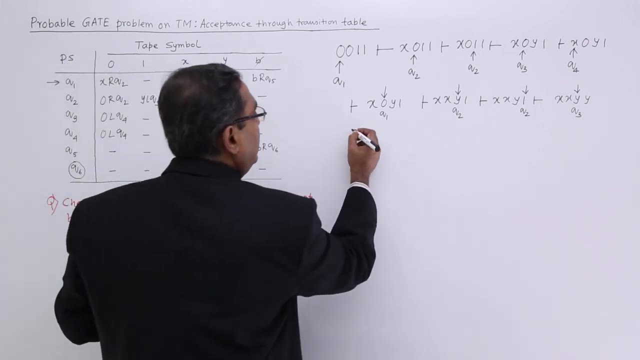 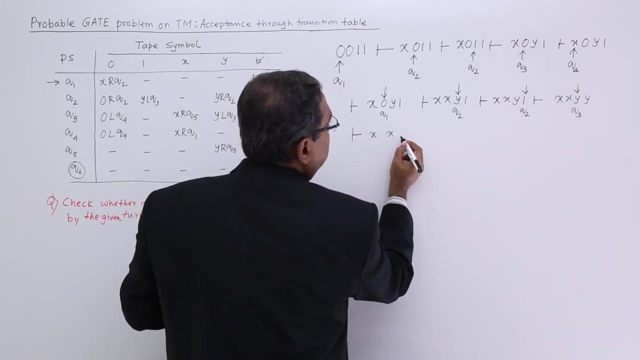 one is Q 3 Y, So Q 3 Y. So Q 3 Y means I will be remaining with Y L Q 3.. So Y L Q 3.. So now see, So it will be X, It will be X, It will be Y, It will be Y because Y L Q 3.. So Y will. 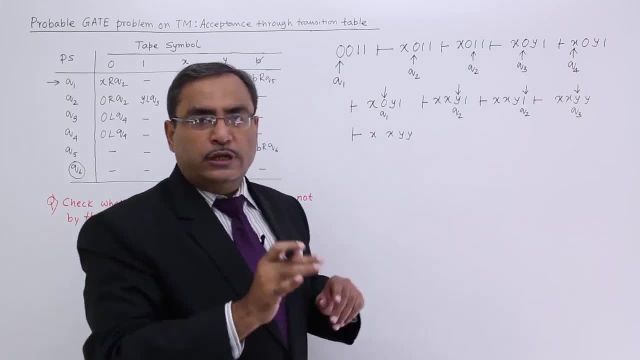 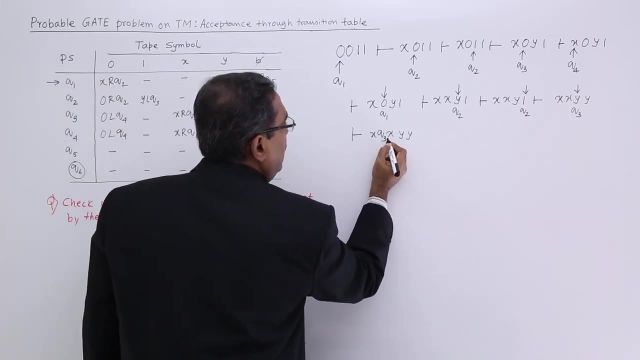 be replaced by Y. It will come towards the left Here. I shall not give any arrow. I shall write this: Y L Q 3.. I think, let me check once- Y L Q 3.. I shall write this state before that very input symbol on which the red red head is there. That means I am moving towards. 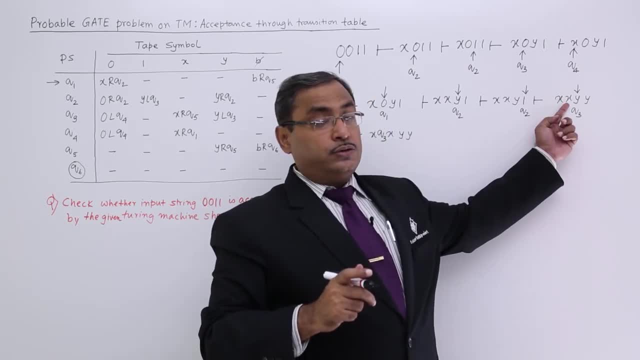 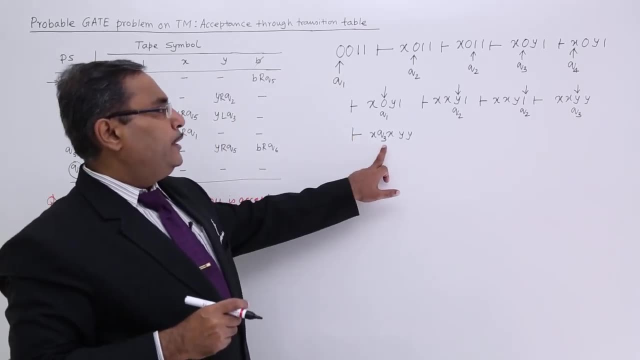 the left. So I am, I will be on this X. So the state next state will be written prior X. So there is a notation number 3.. So here we need not to put any arrows, Not like this, Not like this. But here I will be writing. 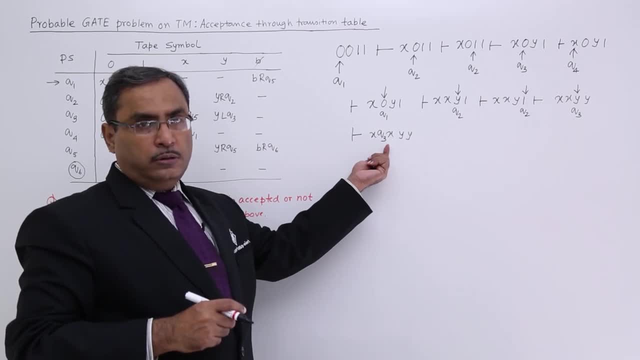 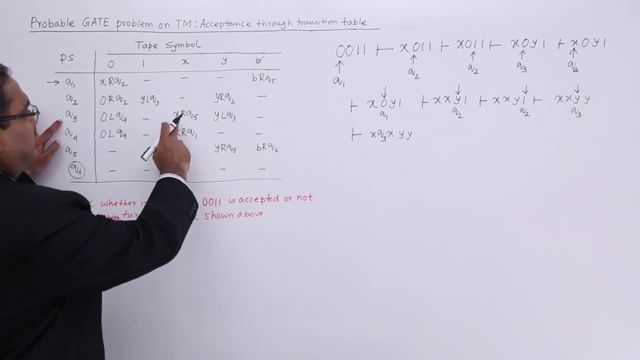 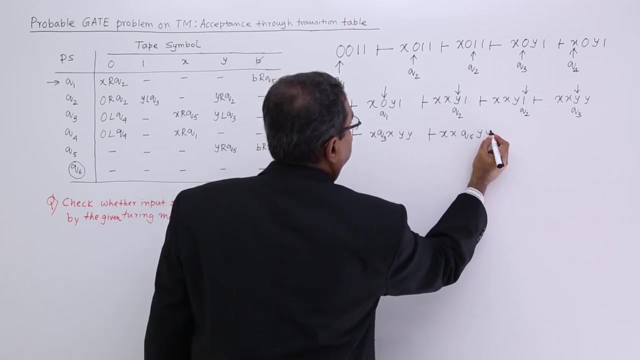 the state before that very particular input symbol on which my red red, red red head is existing Now: Q 3 X, Q 3 X, X, R, Q, 5.. So Q 3 X is X R, Q 5.. So Q 3 X is X R, Q, 5.. So. 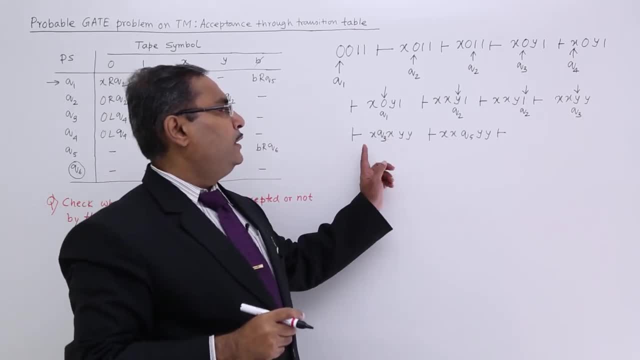 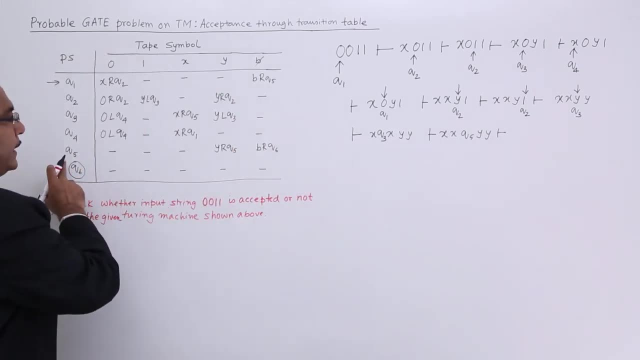 it will be red, So it will go to the right. So it will come to the before Q, Q, before Y. So this one: Q 5, Y, Q, 5, Y. I am going for Y R, Q, 5.. So Y, X, X, Y R, R means right hand. 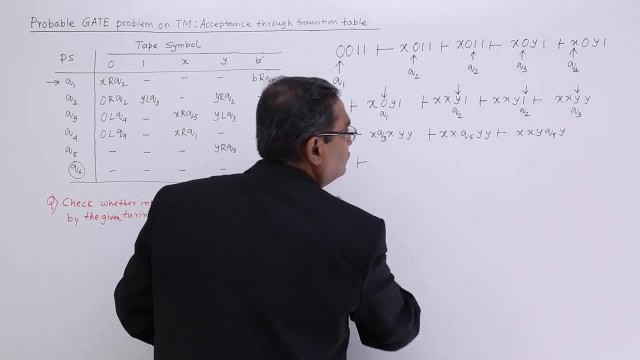 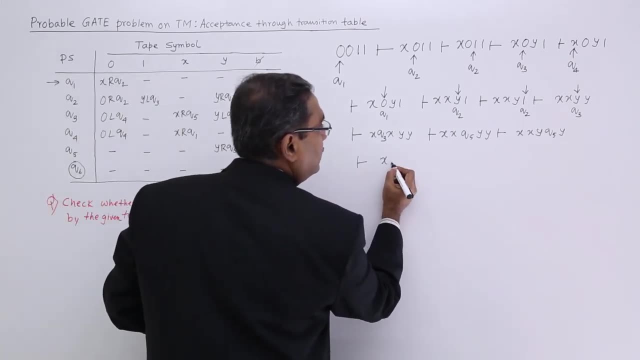 side and Q 5.. Now Q 5 Y Y R, Q 5.. So Q 5 Y R, Q 5.. Now Q 5 Y R Q 5.. So Q 5 Y R, Q 5.. So X, X, Y Y, Q 5.. As it here is nothing, So I can easily write blank. So that is. 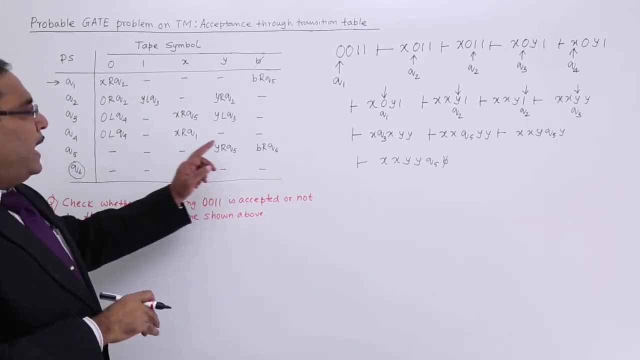 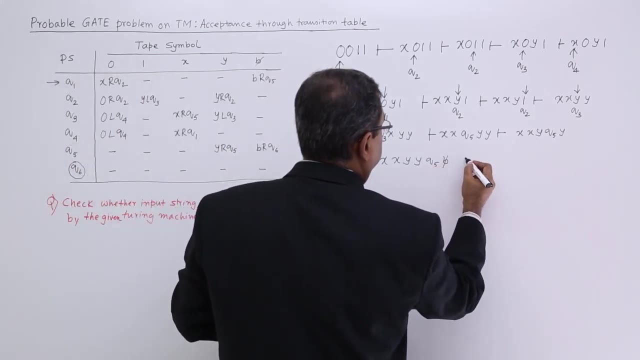 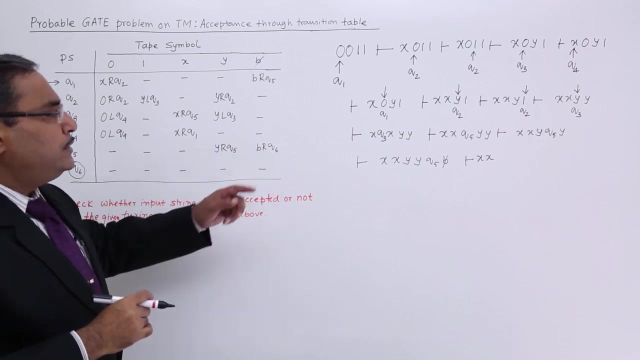 not an issue. I can write blank. So Q 5 blank is blank, is blank R Q 6.. So now Q 5 blank. Q 5 blank. we are having blank R Q 6.. So now I shall go for this. So Q 5 blank is blank. 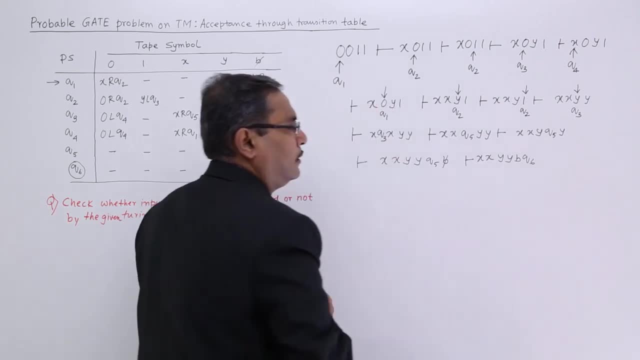 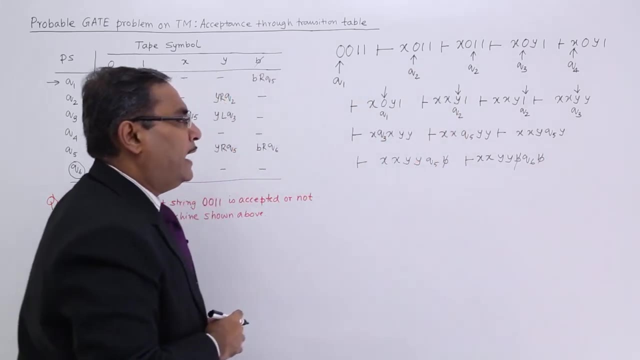 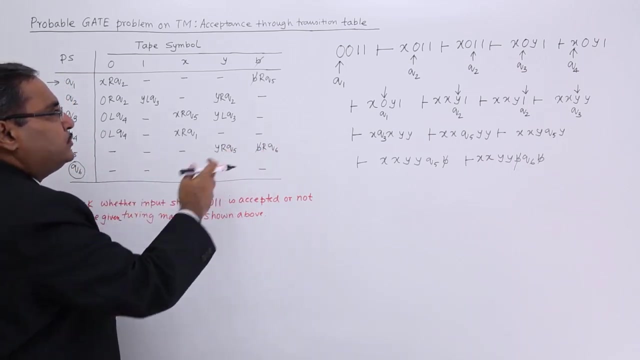 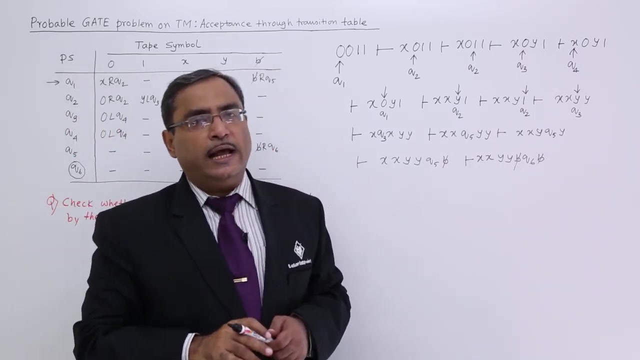 But here you see, after Q 6, that is blank, After Q 6, that is blank. After Q 6, that is blank. So Q 6 against the blank, there is no transition defined, So the machine will halt and as the terminating state, Q 6 is the final state, So the string has got accepted. 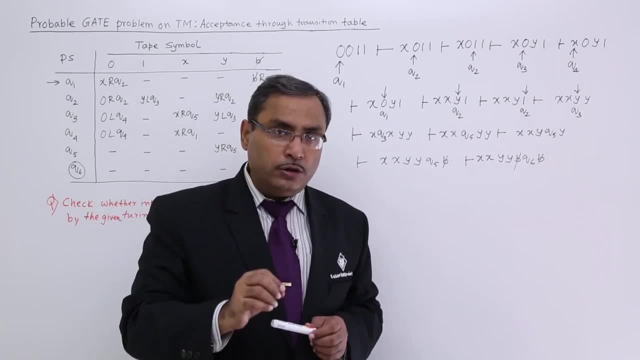 So I should wait until I halt, and if I can halt until then, it is ok. Now, when R 2, I get R 0, and R 3 R 2 or R 3 R 3, I are left to in this order Then. so next this run could. 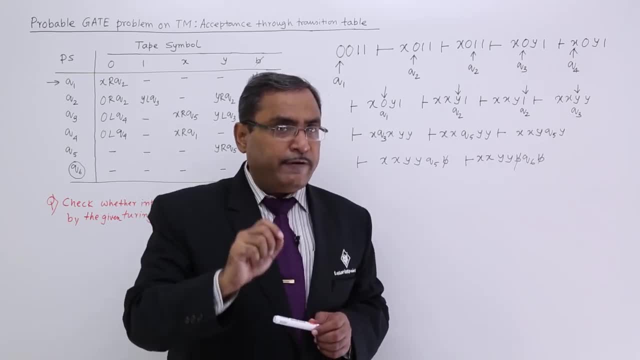 be what P? r after R, R, Q, 6.. Then I would continue and even again continue, until both of them- The does add, differ in the terrible of me. And so now you are exactly what the machine can do to. then I shall check what is the terminating state, is it a final state? is it so? yes, then, 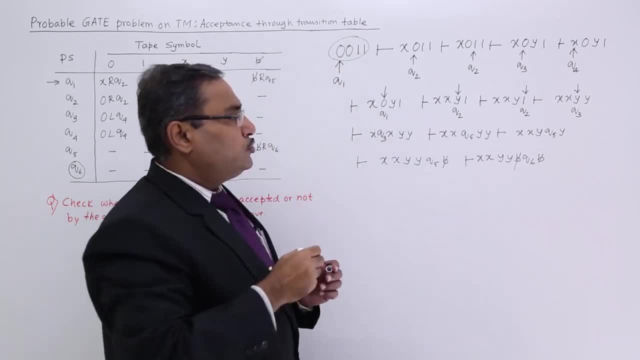 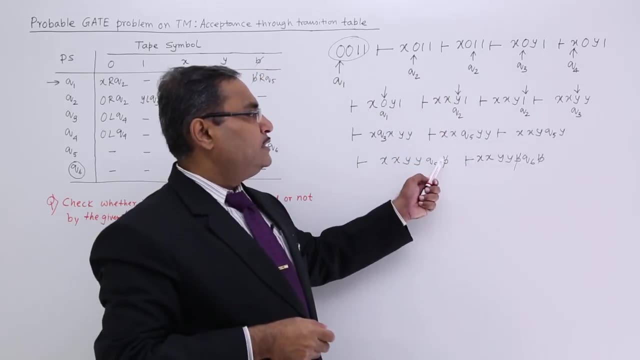 the string will be accepted. which string this string will be accepted. So in this way I have solved this problem. So I have shown you 3 notations: notation number 1, notation number 2 and this is my notation number 3.. So any notation you can use in your exams. thanks for watching this video.